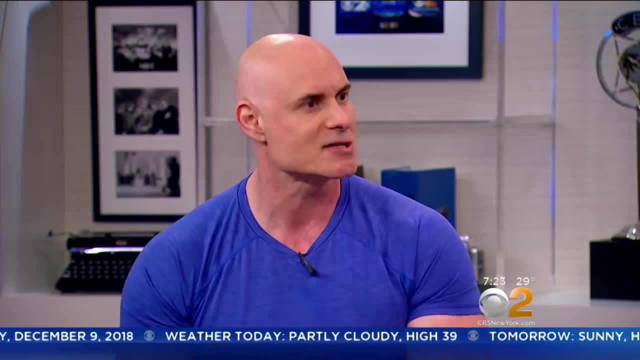 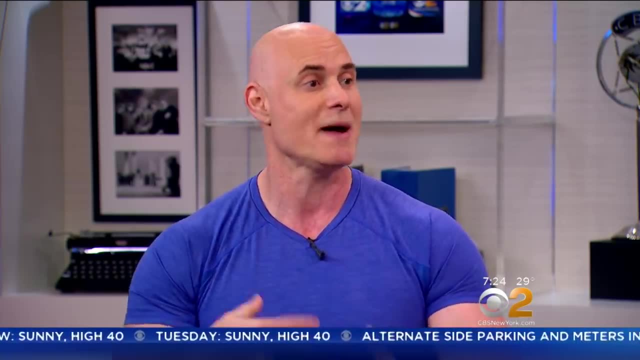 a book called The Captain's Corner And in Captain's Corner they talk about how the kids can become fit and healthy. All of the characters in the book and all of the lessons that were in that particular issue will basically go back and help the kids with specific exercises. 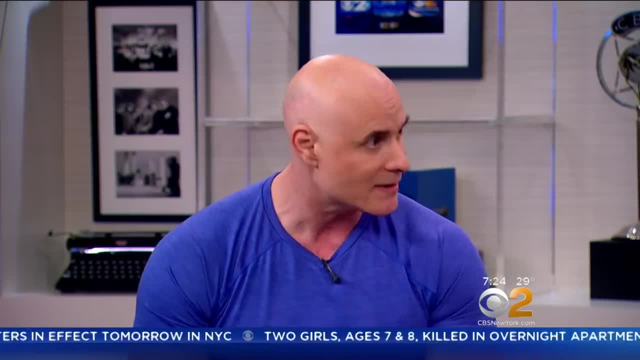 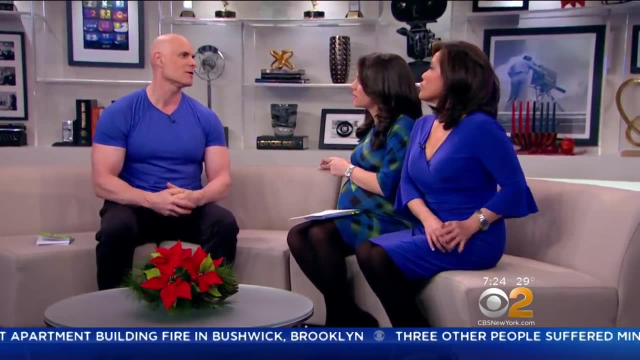 Because you really have to do three things: Kids have to be very good at running, They have to be very good at strength And they have to be good at flexibility. Running, strength and flexibility- Right, right, right. So the running is important because you want to create an oxygenation, You want 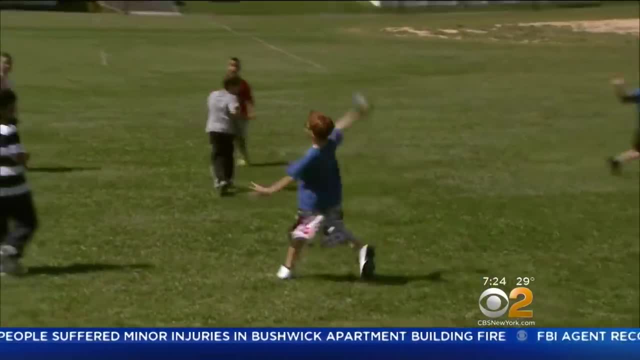 to get the body exercising. You want to increase blood flow and all that kind of stuff. So you want to get the body exercising. You want to get the body exercising. You want to get the body exercising, And then you want to make sure the kids are strength training because you want to build. 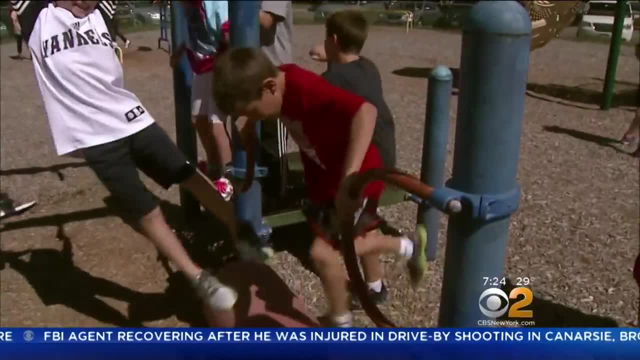 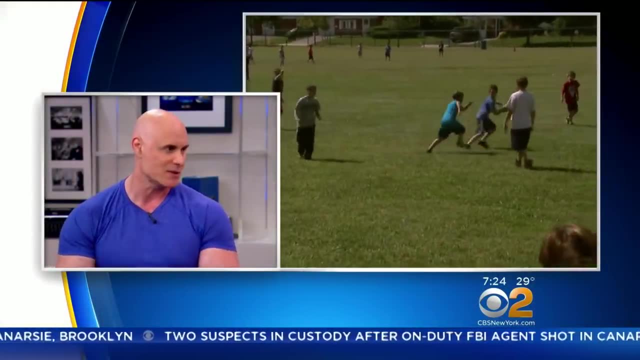 strong muscles And you want to make sure the bones are strong as well. Don't forget, a child will keep growing up until the early 20s And those long bones won't actually fuse until the early 20s, So you want to keep them exercising that way at an early age. Learn the lessons early. 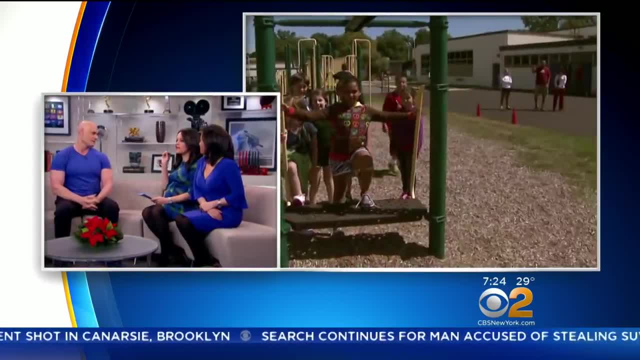 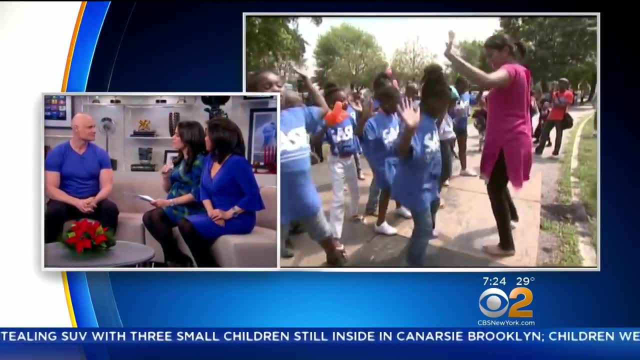 And, of course, eating well. I was just going to ask you, especially this time of year where there's sweets and all sorts of stuff and parties, what is your best advice for parents who do want to try to get their kids to eat healthy? eat those vegetables and their fruits and everything. 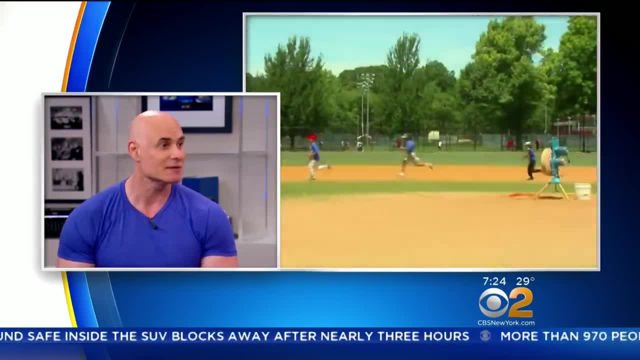 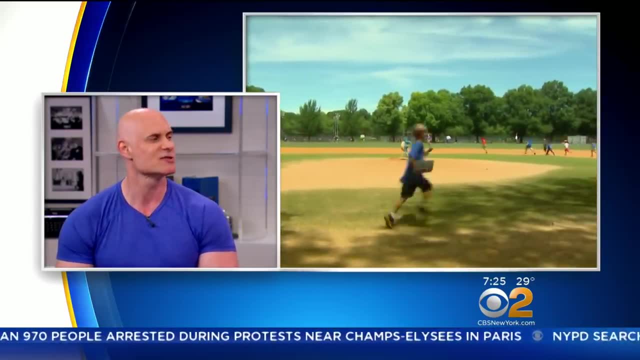 Get them involved in the process of creating the food, of making the meal. If you give them a little job to do, they'll be more prone to maybe want to eat their own creation. Another thing that you can do is kind of fool them a little bit by adding fruit to something specific like a salad. 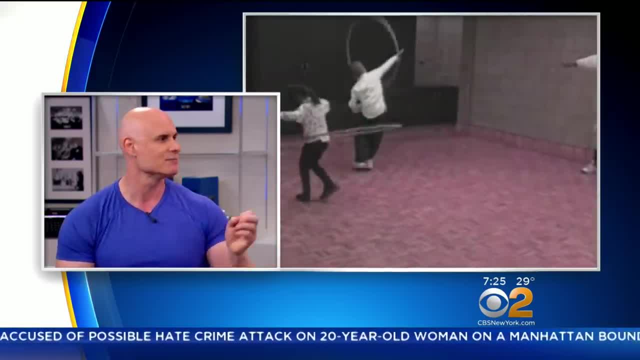 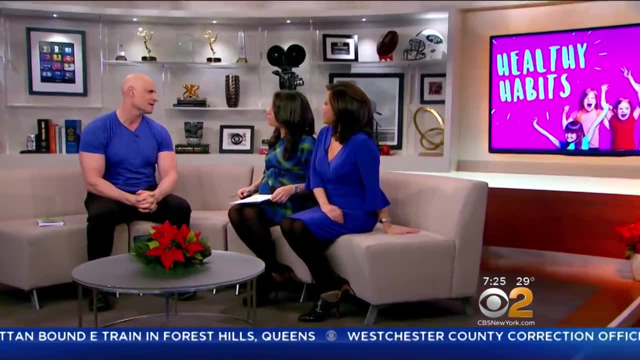 Take your salad and chop it very fine and then add some apple and some pear and maybe top it off with a little bit of raisins, because you're getting good nutrient value in raisins. in your time I know you train a lot of kids in different sports and things. What would you say to parents? 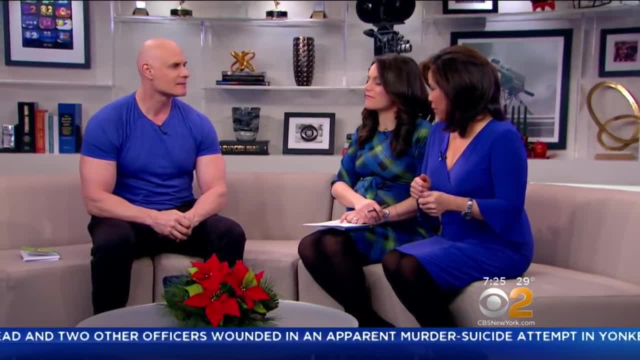 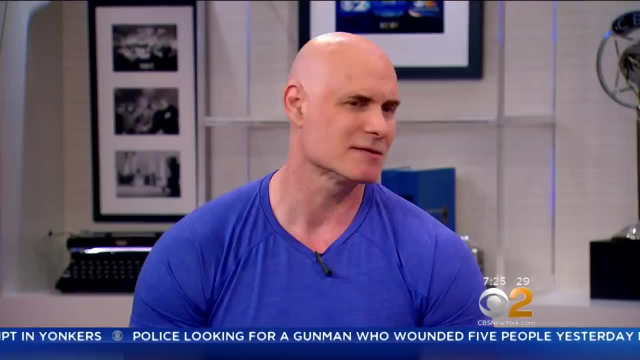 who might have a child who's just always like this and always on the computer and it's hard to get them started If they're not already in a sport or something. how to really motivate them? It's hard because right now kids are always watching a screen of some kind. If we can limit. 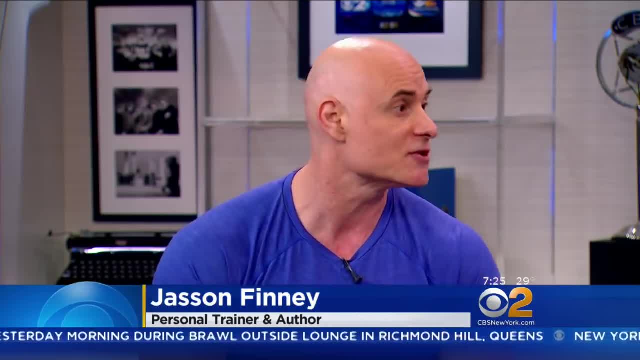 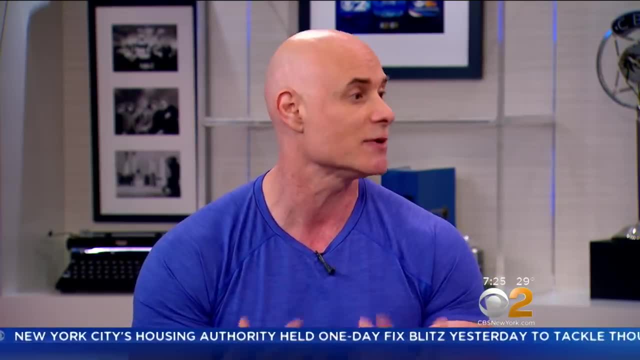 the screen time. that'd be fantastic. How do we do that? Get involved with the child, Make it play time, Make it fun. Kids love to use their imagination. It's all about exercising through what they can create. If they can't do it, they can't do it. If they can't do it, they can't do it.